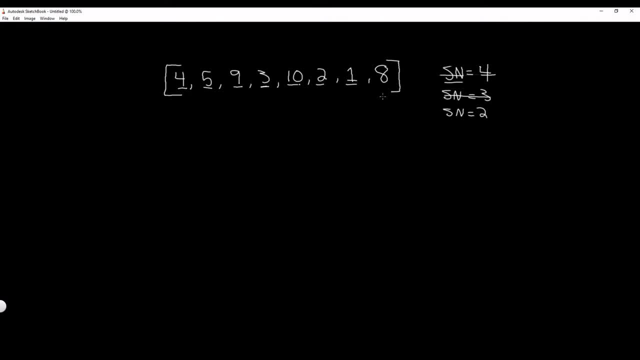 Then we go to our next item. Is 1 smaller than 2?? Well, yes, it is. So we update it again: Smallest number is equal to 1.. And then we go to the next item in our list. Is 8 smaller than our smallest number? Well, no, it's not. And now that we've iterated throughout each item in our list, we are done. So all we have to do from here is return our smallest number variable, which is 1.. And it's going to give us the smallest number. 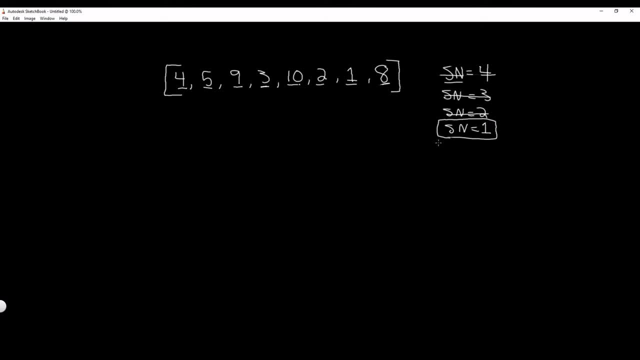 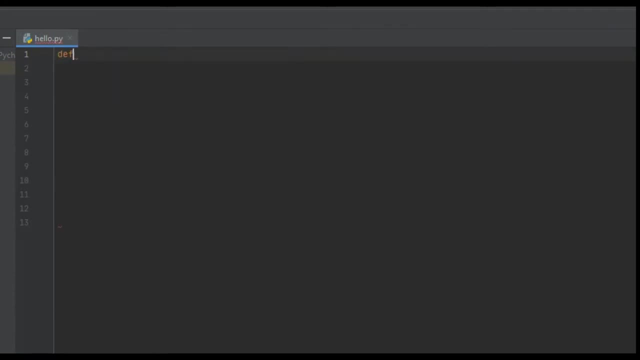 So that's basically how this smallest number algorithm is going to work. Stick around for the next section of this tutorial to learn how to code it up. So for the coding section of this tutorial, we're going to start off by creating a function and we're just going to call it smallest number, And then we're going to pass it our list and we'll just call it numbers for now, And then from here, we want to create our smallest number variable. 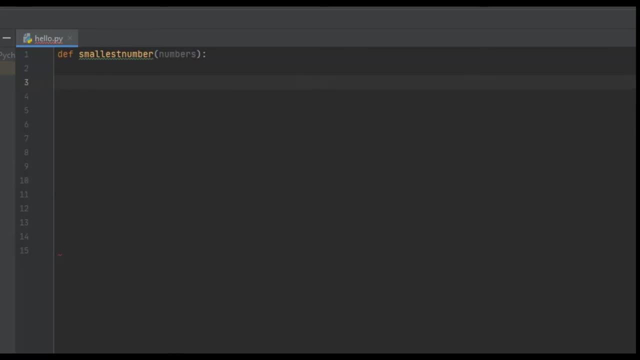 talked about in the algorithmic section of this tutorial. we're just going to set the smallest number equal to the very first item in our list. so we're just going to create a variable called smallest num and we're going to set it equal to the very first item in our numbers list. and we're going to do it. 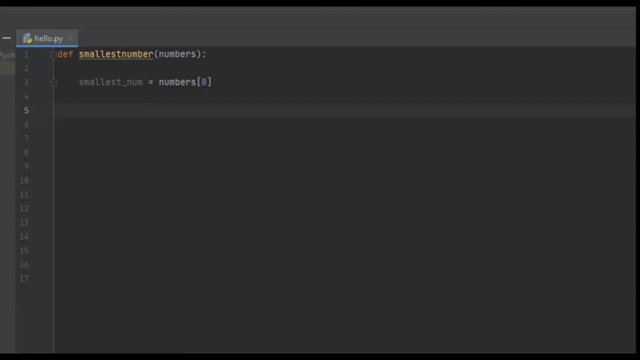 just like that. and now we're going to want to iterate throughout each item in that list. so we're just going to say, for num in numbers, we're just going to check if the current iteration or the current item is smaller than the smallest number. all we're going to do is update the smallest number with that new. 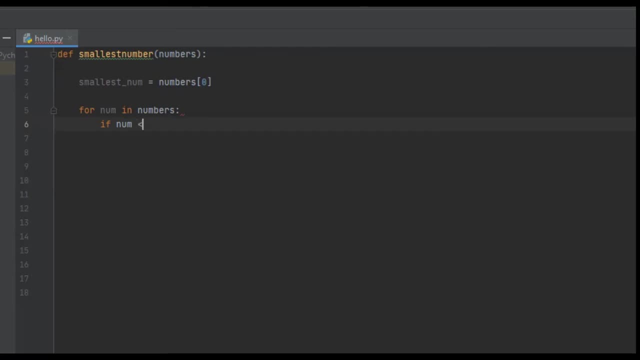 smallest number. so we're just going to say: if num is less than the smallest num, also we're going to say: is smallest number is equal to number and then from here all we have to do is return the smallest number. so we're just going to return smallest. 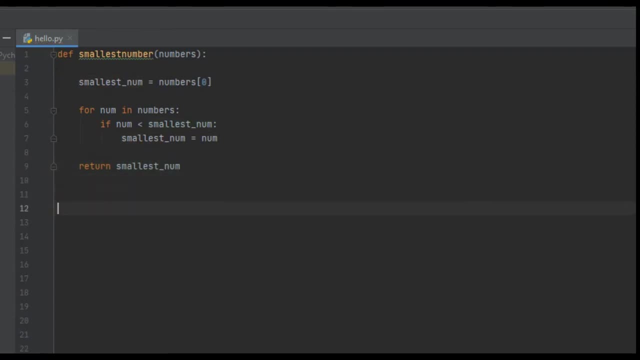 number and then to test it out, we're going to create a function call of the smallest number and pass it a list. so we're just going to say smallest number and we're going to pass it some list of arbitrary numbers. so we're just going to.